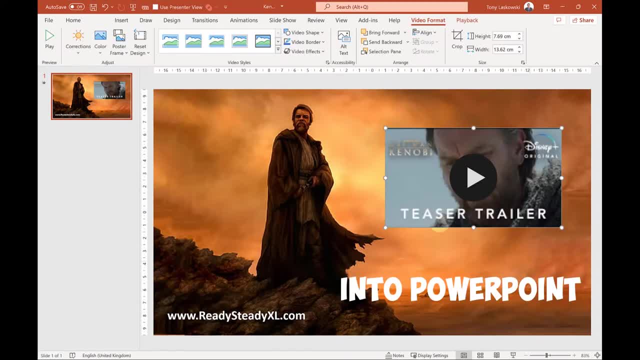 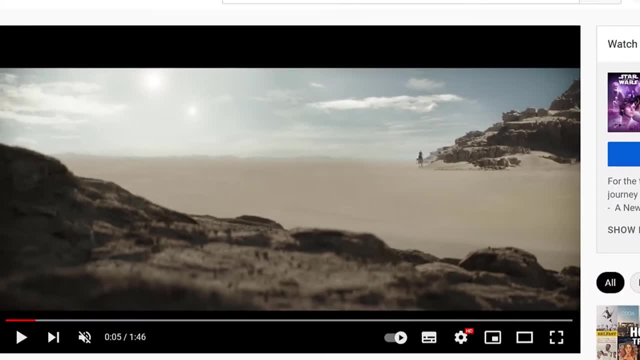 In today's video, you will learn how to insert a YouTube video into a PowerPoint presentation, how to change the cover image of the video and how to get it to play automatically. Here I have the YouTube video that I want to insert into my PowerPoint presentation. 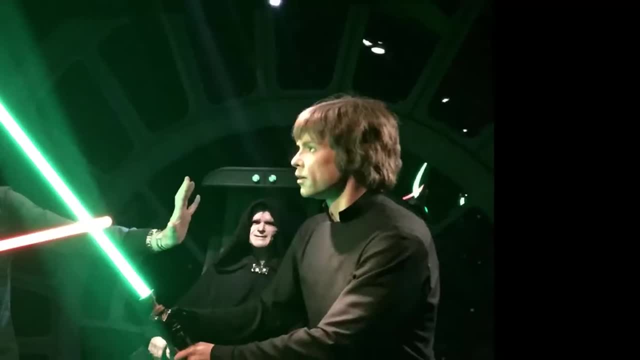 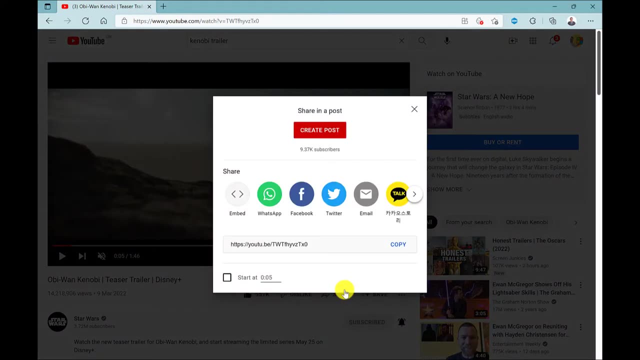 It's the trailer for the new Star Wars series Kenobi. I'm a big Star Wars fan, so I'm quite excited about it. Before I insert this video, I need the URL To get this I go to Share. If I want the video to start from the beginning, I can simply click Copy. 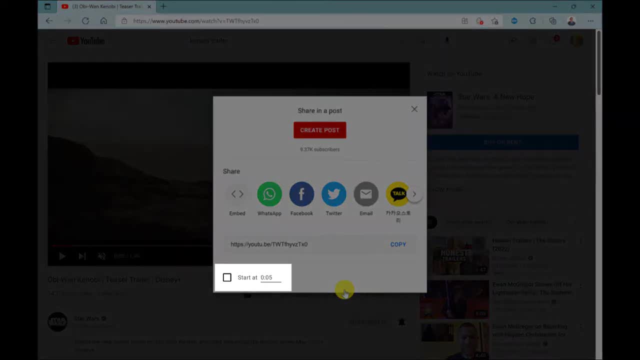 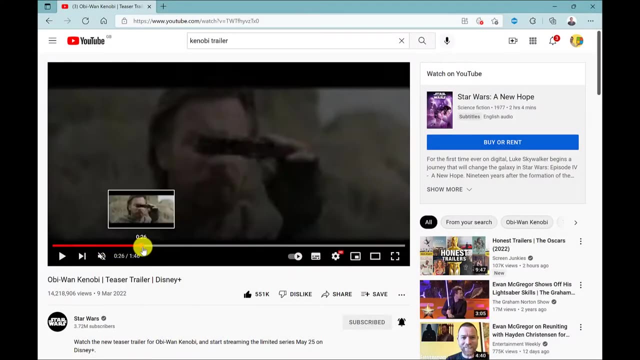 You have Start At. if you want to specify when the video plays from, You can add this manually by clicking here, or an easier way is to drag the timeline to the time you want. So here I'm dragging it to 29 seconds, and when I go to Share. 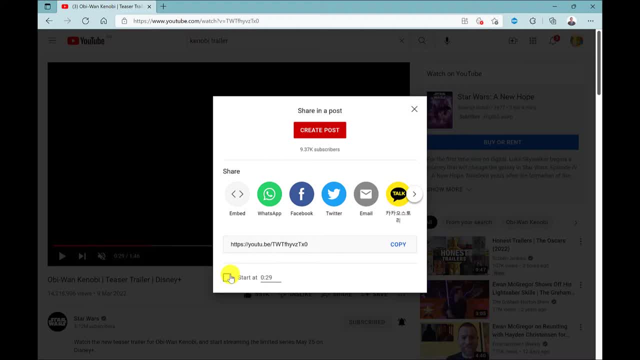 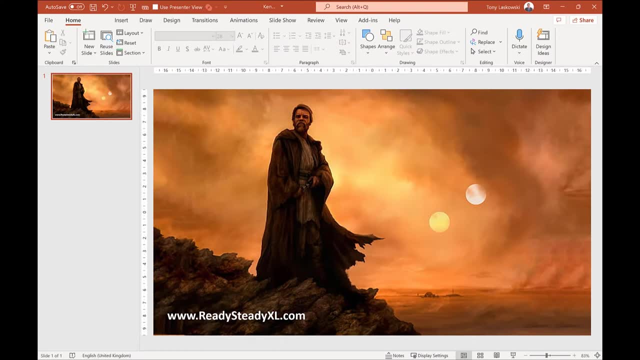 you will see that Start At is 29 seconds, So I click here and then select Copy. Next go to your presentation. Here's one I've prepared earlier To insert the YouTube video. I go to Insert over here to Video and select On-Return. 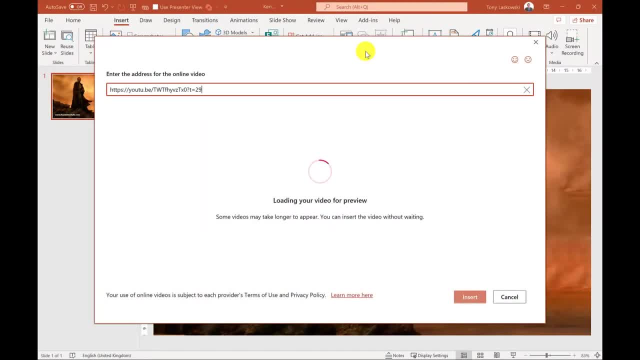 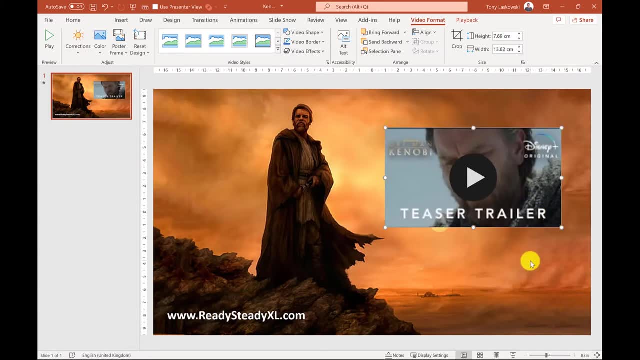 I'll paste my URL into here and when it's ready to be inserted, you will get a preview video. This video can be positioned and resized To change the cover image for this video under the Video Format tab, which will appear when the video is selected, go to Poster Frame. 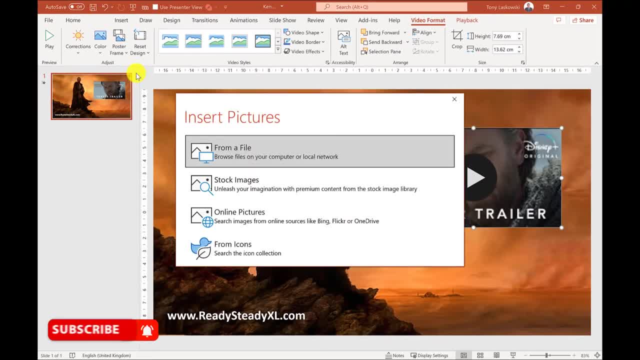 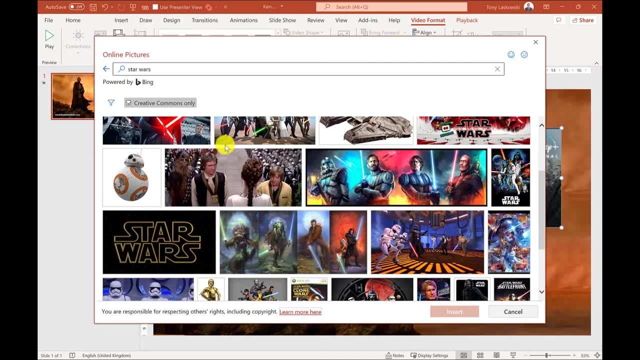 select Image from File and then select your image from one of these options here. In this example, I'm going to Online Pictures and I'm going to search for Star Wars. I select the image I want and then click Insert and the cover image for the video updates. 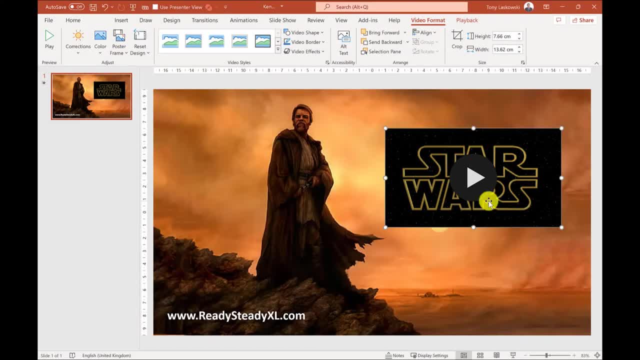 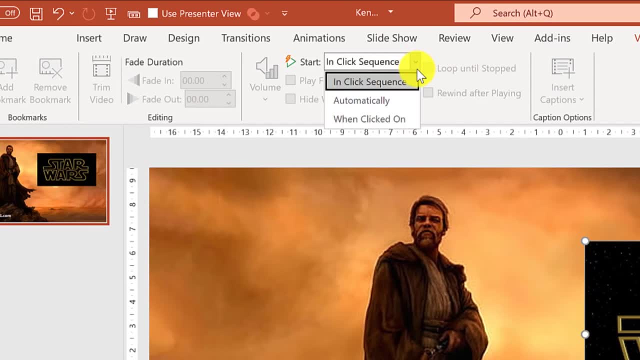 If you want this video to play automatically in your presentation when you go to this slide, then go to Playback. A lot of the options are greyed out, but if you go over here you can select Automatically When I start my presentation. 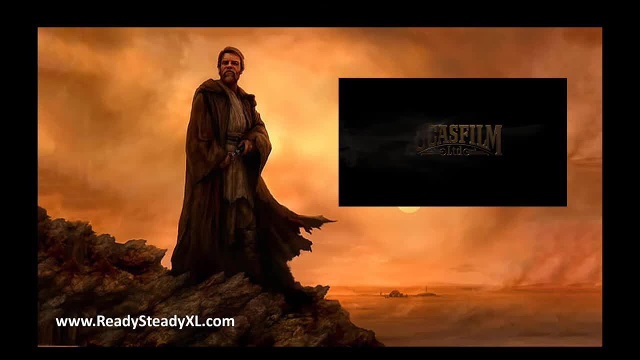 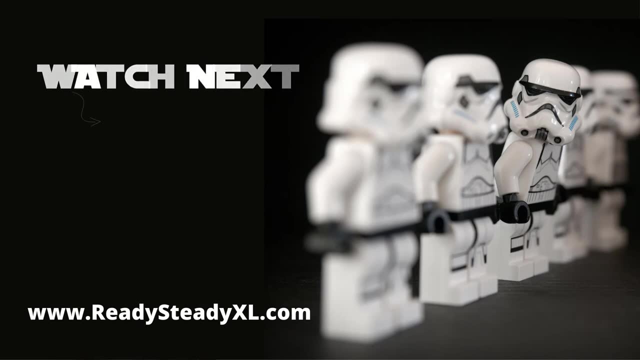 the video will start to play automatically. If you want the audio to be heard in a Teams meeting, then watch this video here. and may the Force be with you. So I'm going to save my presentation and I'll see you in the next video. Thanks for watching. 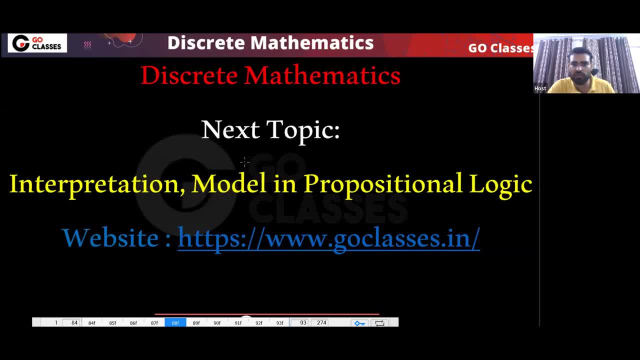 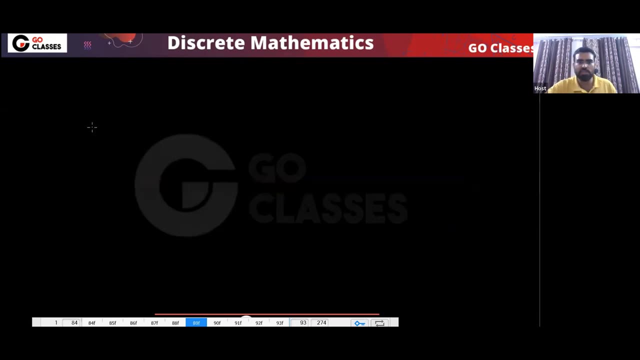 What is interpretation and model in propositional logic? So first we will study about propositional logic. Okay, so first remember we are only discussing for propositional logic first, After that we will discuss for first order logic. So interpretation, comma model in propositional logic.